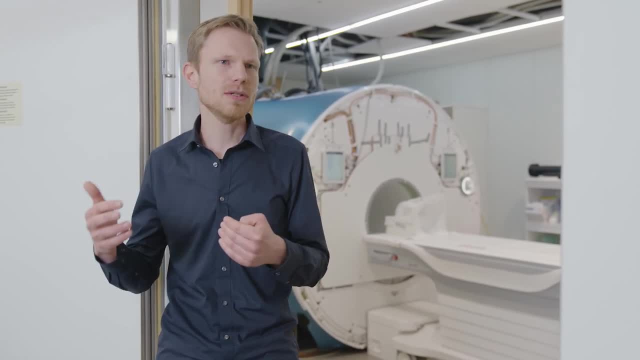 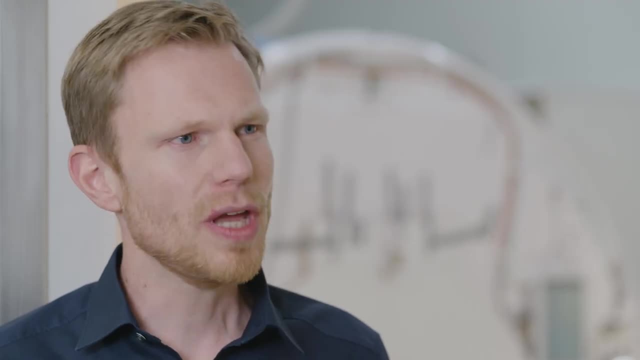 However, with standard technology, a further increase of the gradient strength would lead to reduced speed by which the system could reach its power. So with the new technology we aim at both large gradient amplitudes- so large gradient strength- and short ramp times- so high slew rates. 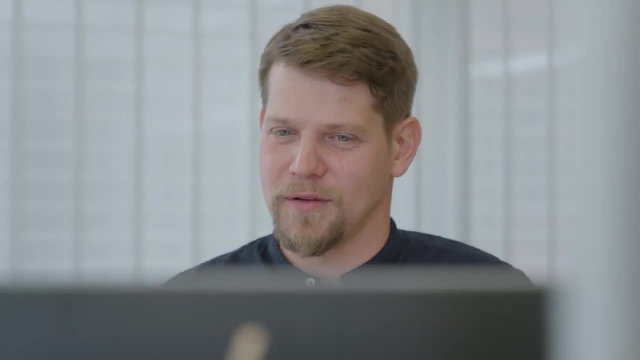 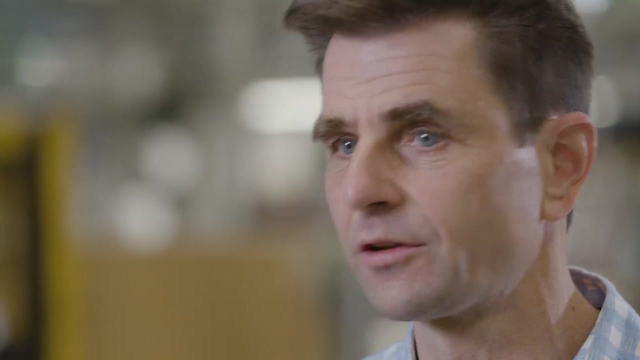 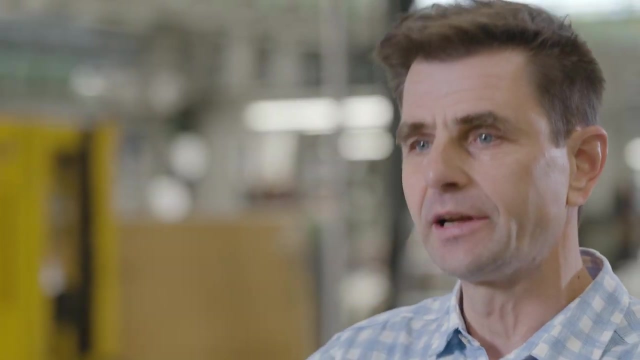 We start with a concept design that has all the ingredients to generate the ideal gradient field, And this design then turns into a design which accounts for all aspects of the real world of manufacturing. The idea is not just to increase it slightly, but to make a significant step in the available gradient strength. 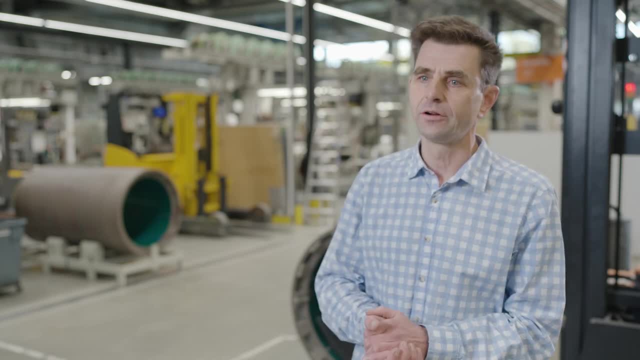 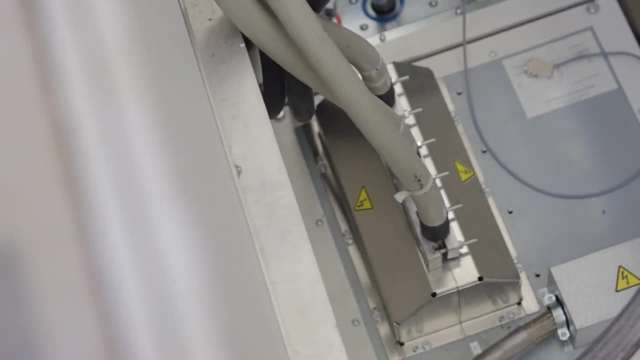 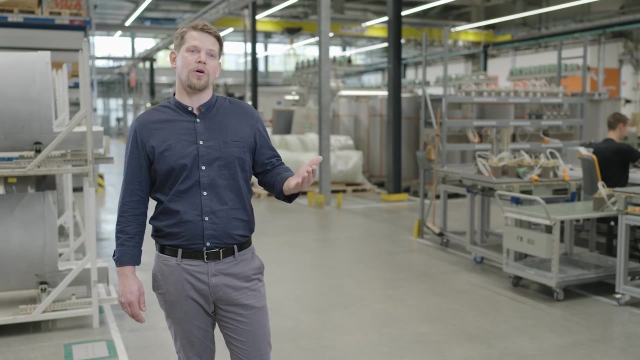 We achieve this step by using a new technology, a double GPA technology. It means we drive our gradient coil with two gradient power amplifiers. The main challenge is to enable the multi-GPA technology. Therefore, we have to divide the gradient coil into two separate circuits. 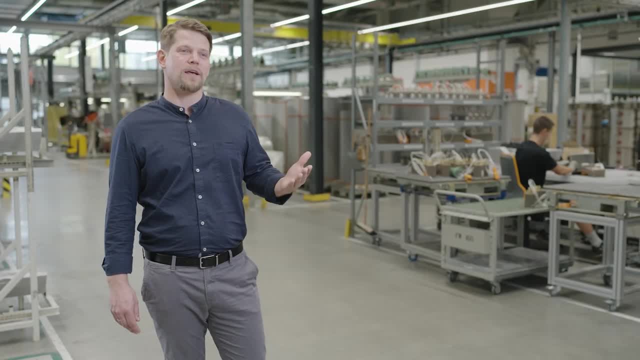 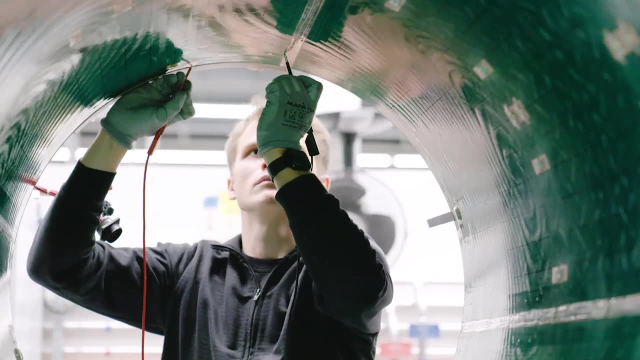 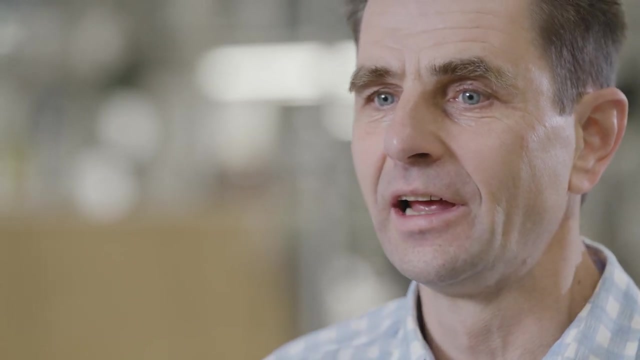 Due to this requirement, we doubled our set of interfaces and electrical connectors, which result in a very complex layer structure. It's so difficult because space is limited, And the more field we want to generate, the more conductors we need, And so we have to find a compromise between available space. 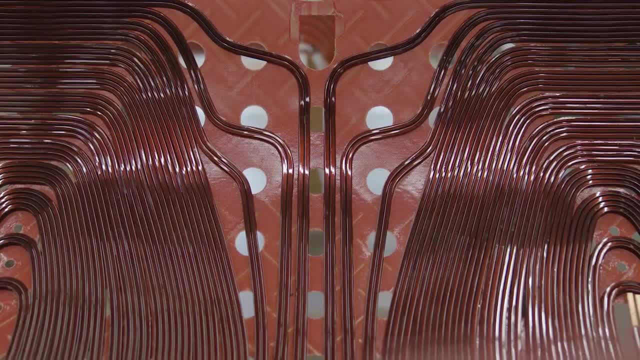 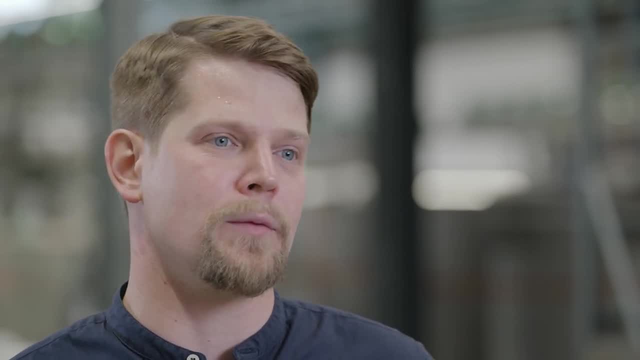 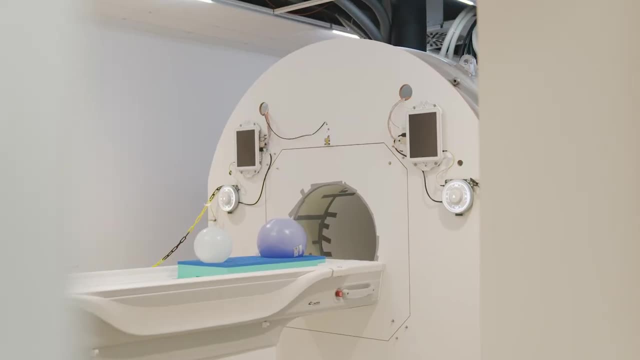 and the ideal aspects of an ideal grain coil. Another difficulty always is to translate the physical design concept into a manufacturable product, Because a manufacturable product always has far more requirements than the physical design concept. Usually we have only one GPA for one gradient. 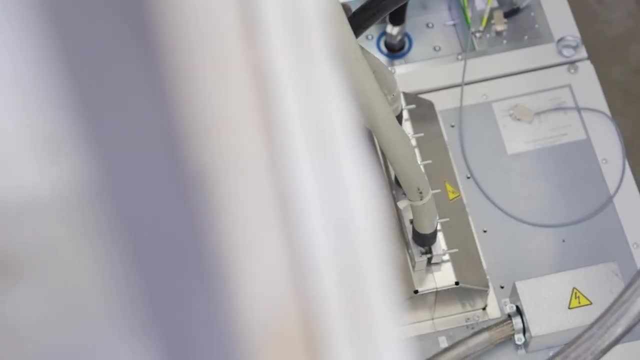 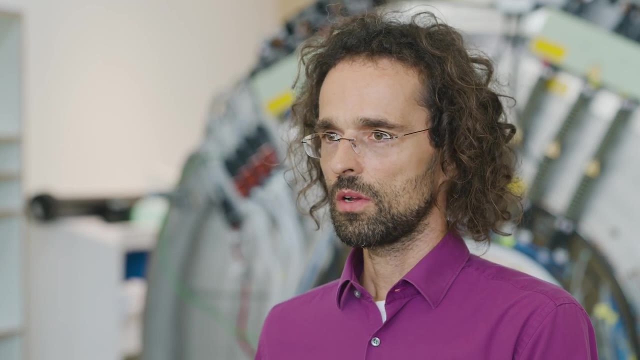 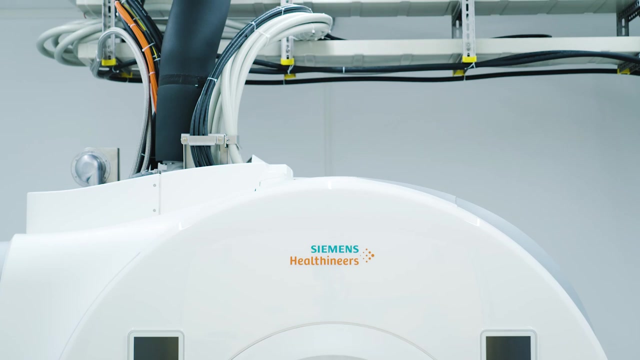 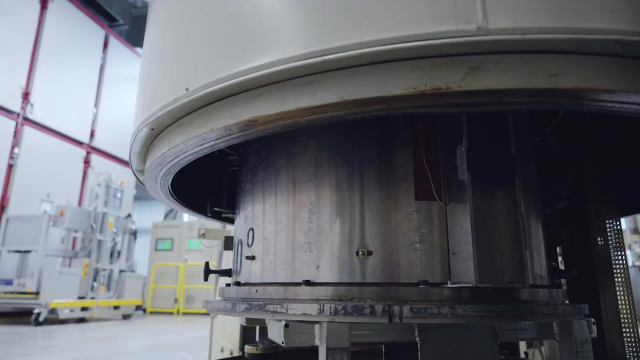 The idea now is to have two individual GPAs Supporting and controlling two separate parts of the same gradient coil. This would allow us to increase the speed at a given power so that we would have a maximum speed at maximum power. The main challenge was to truly synchronize both GPAs.